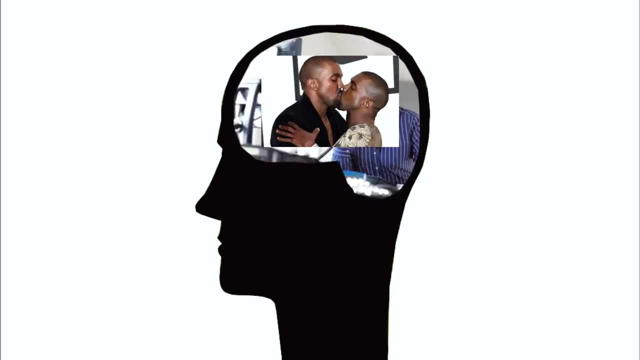 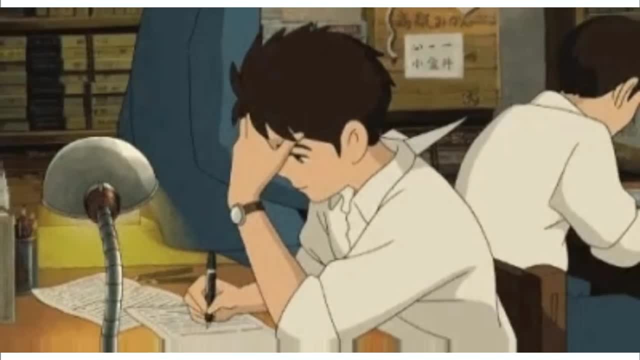 challenge And it had me using 20% of my brain power trying to solve this problem, But at the time I was still having fun with it. It was still easy while also having a little challenge. It's like video games. 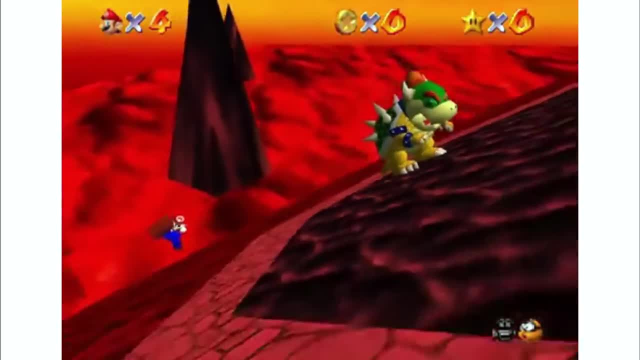 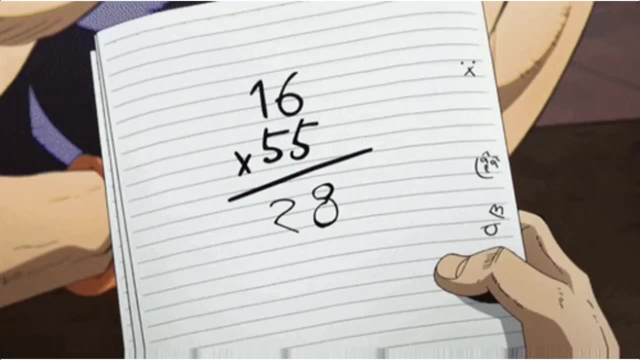 You don't want them to be too easy all the way out. You want little challenges scattered throughout the game to keep it interesting. That's how I felt learning addition and subtraction. and I felt that even more when learning multiplication. Bruh, doing multiplication back then was so fun. 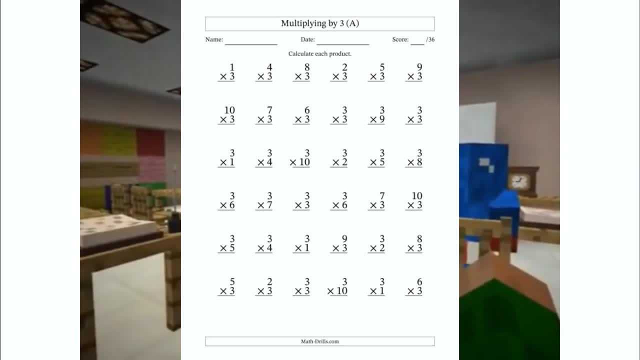 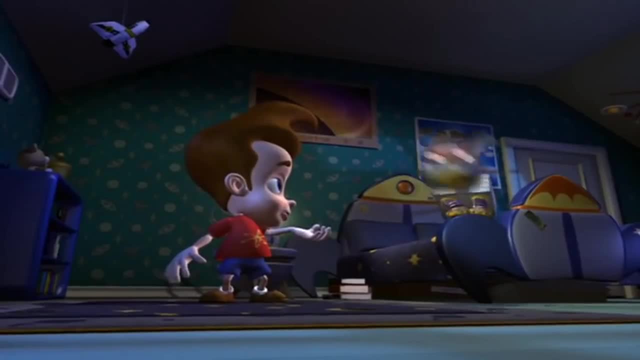 I was a multiplication god. Whenever I was handed those 50 question multiplication sheets back then in elementary school, I would speed run that in 5 minutes or less and get everything right. I felt like Jimmy Neutron, the boy genius, Except I had a bigger head. 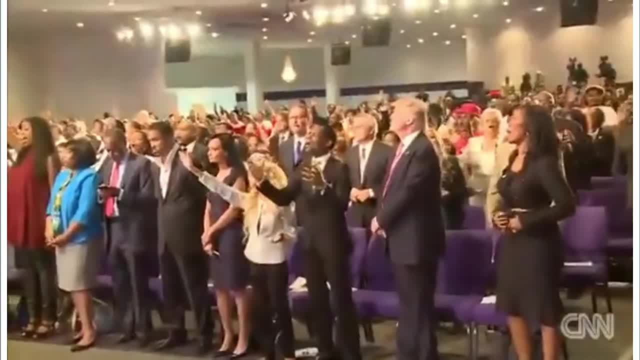 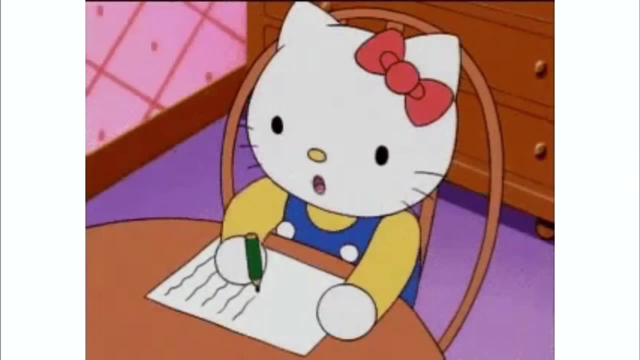 Multiplication was so fun that I would legit be doing it during my free time. I remember one time I was at church and I got bored because it was church, So I pulled out a notebook and wrote down a random multiplication problem. I ain't even. 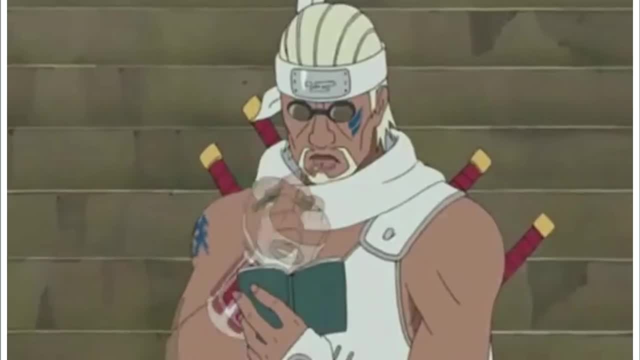 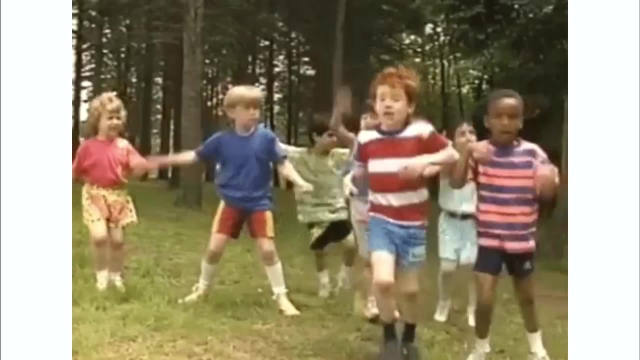 know 16 times 16.. I spent the next 10 minutes solving that problem with no calculator and I got 256.. I was so smart man, What up. What other 3rd grader knows 16 times 16? out the jump other than me. 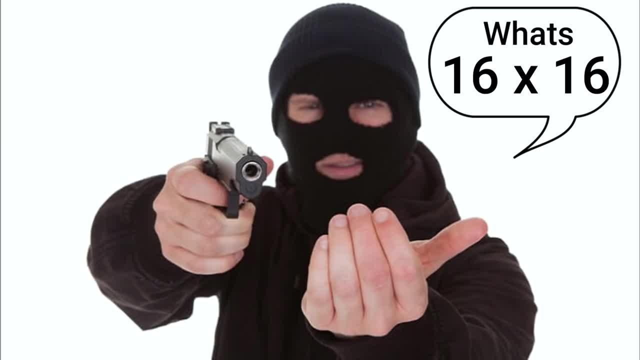 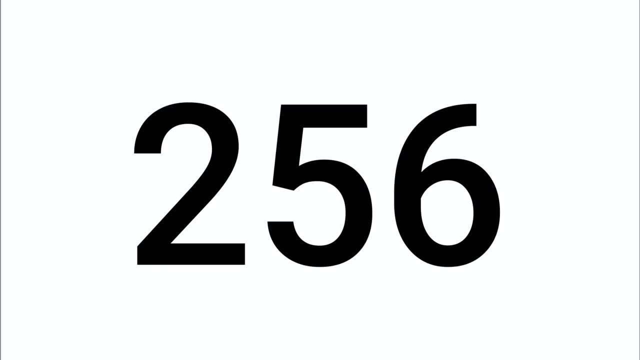 Someone could have a gun to my head and tell me what 16 times 16 is. You have 2 seconds to answer. 2 seconds, Man. I'll answer that in 0.2 seconds, 256.. Ain't, nobody could solve multiplication like me. 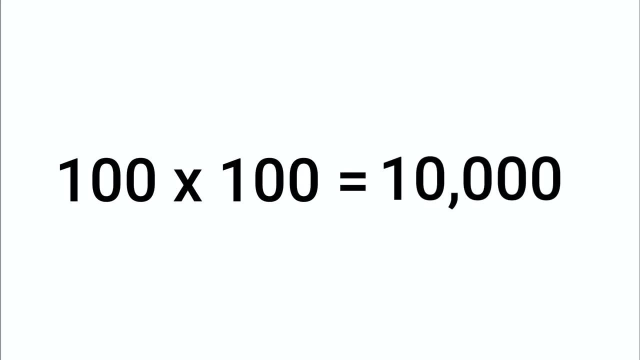 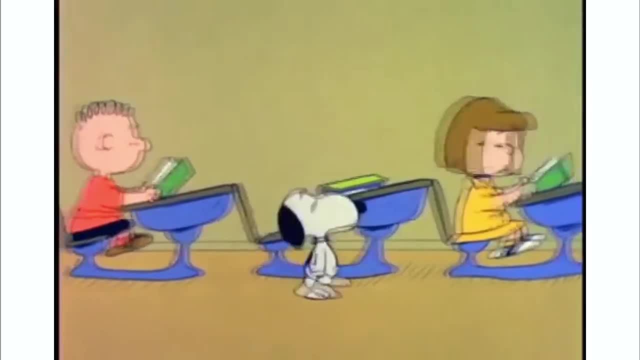 I'm the multiplication god: 100 times 100? 10,000.. 10,000 times 10,000? 20,000.. Man, I'm like Albert Einstein When math was like that Simple and easy to understand. 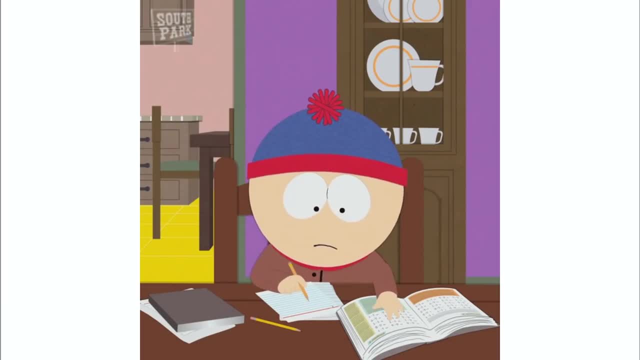 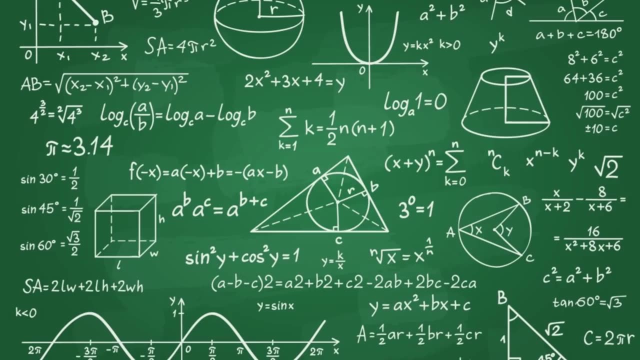 It was fun. I loved that kind of math. So to the person that created those basic math formulas, thank you, And to the people that created everything else, you could suck a HORSE COCK After multiplication and decimals. math was never the same again, because they started. 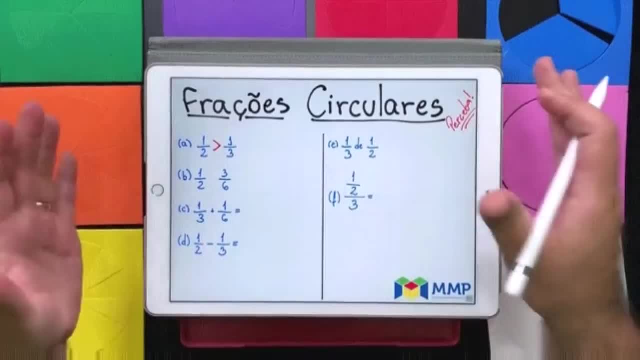 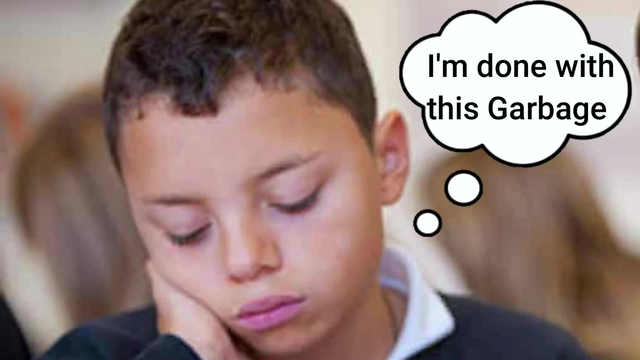 adding all this extra shit. The decay started with fractions. Fractions were easy at first because I was just converting them to decimals to get the answers, But then they started asking for fractions as answers And I was like I just can't do that. 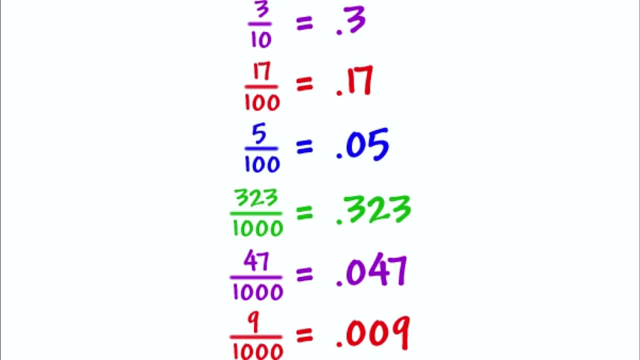 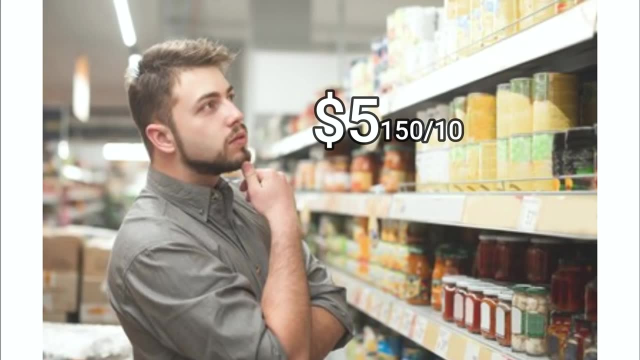 That's not how my brain operates. I convert numbers to the shit I actually see in day to day life. If something costs $20, I'm not going to be like that- cost $5, $150 over $10. I'm not going to be like that. 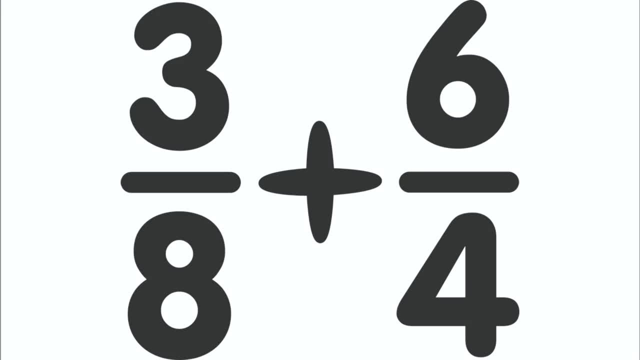 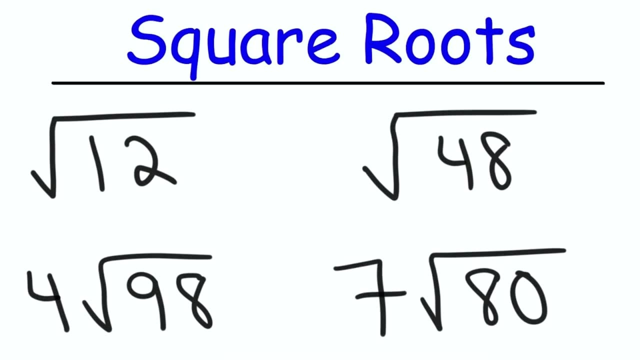 Why do I have to put this in fraction form when I put the same answer in decimal form? You're making this harder on purpose, And it continued to get harder and harder. with graphing, square roots functions Like: is this even math at all? 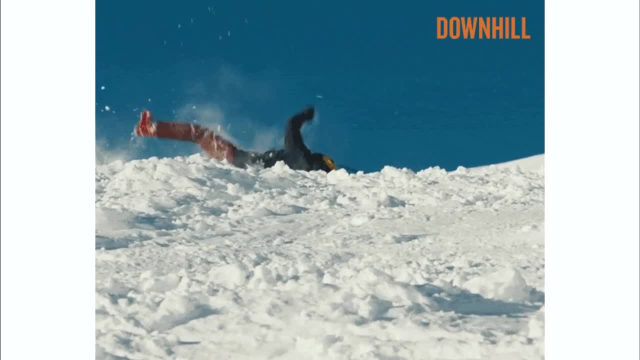 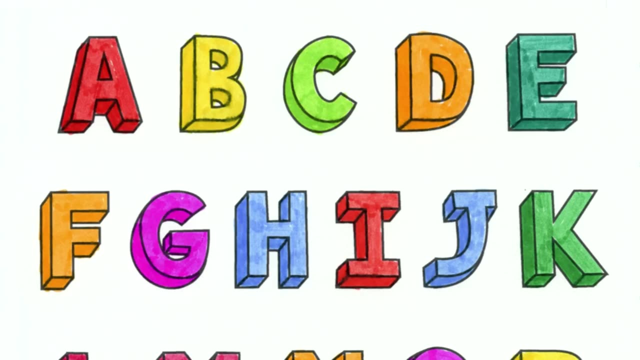 I don't know, And it just hit a slump when they started adding letters to math. Letters are in the alphabet, They're not numbers. Why are they in equations? This shit don't add up. Who did this, Fran Fran? 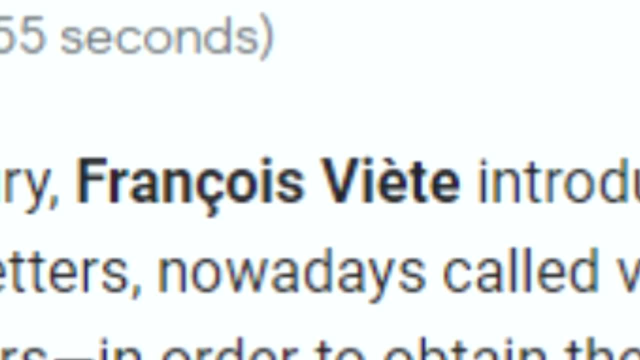 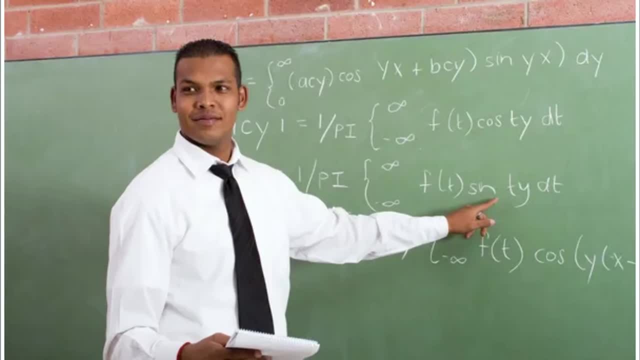 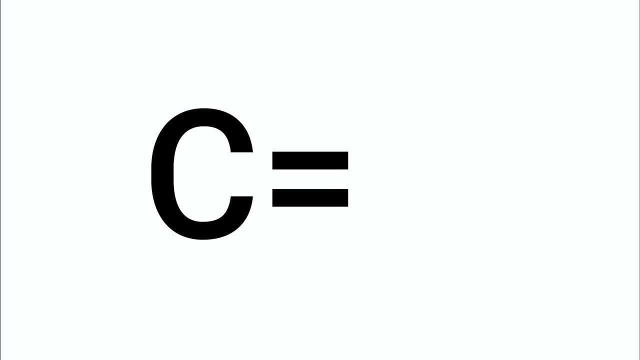 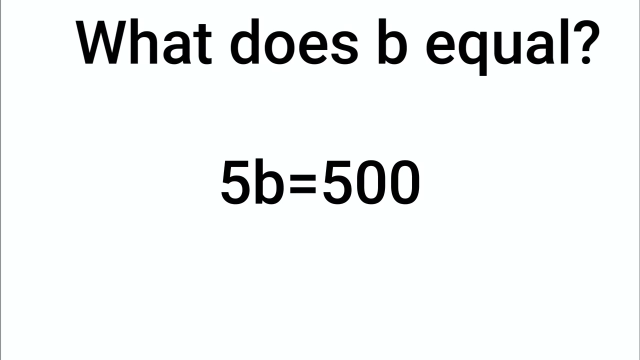 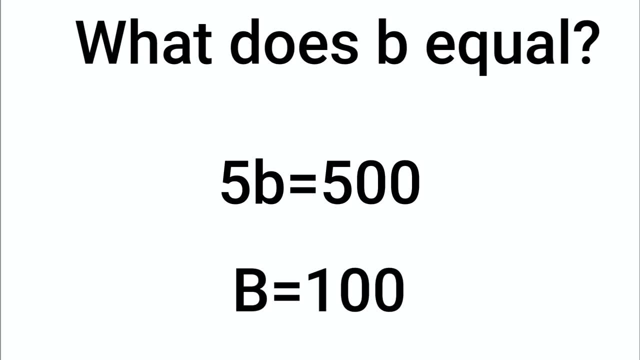 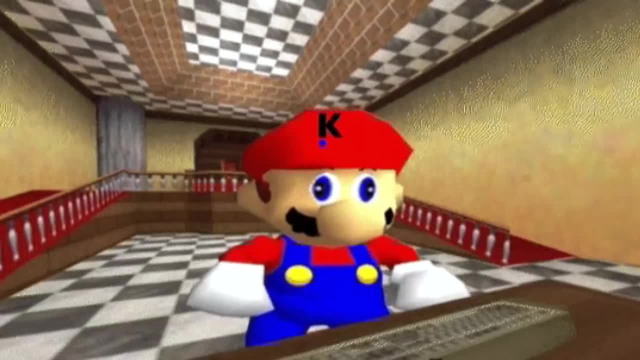 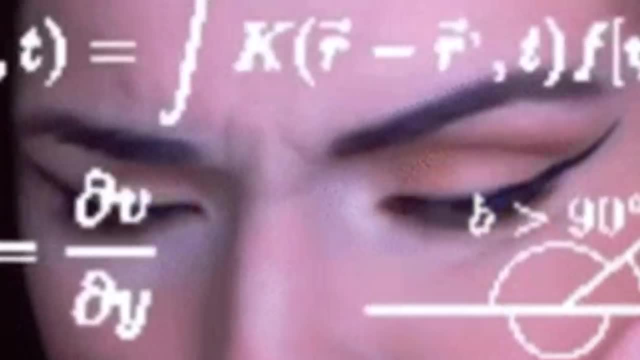 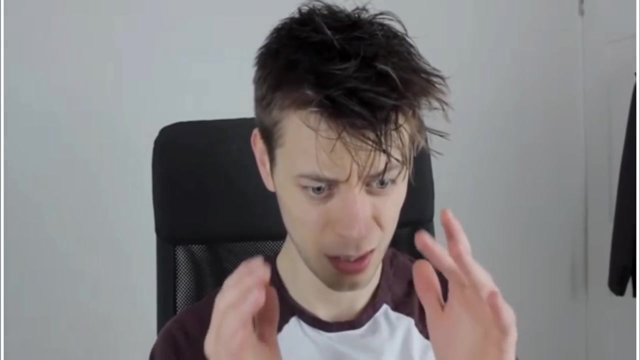 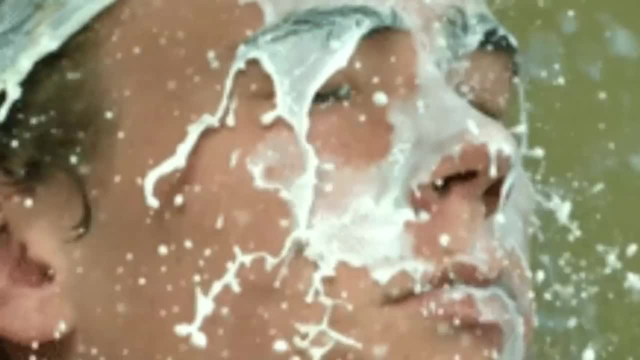 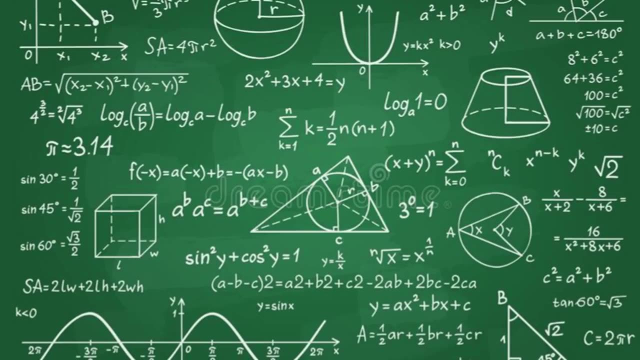 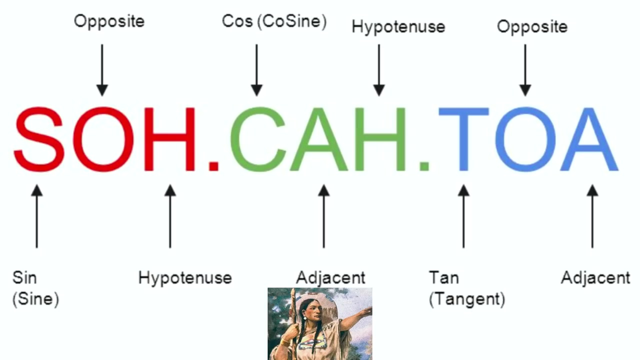 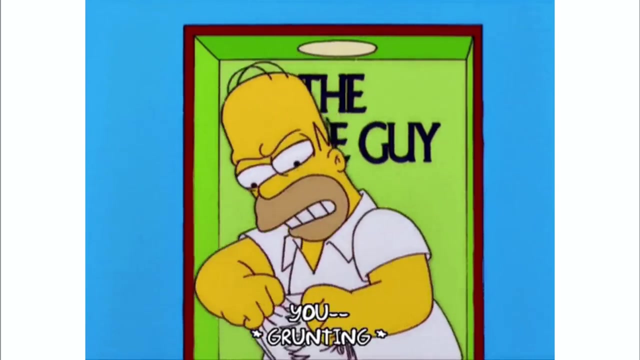 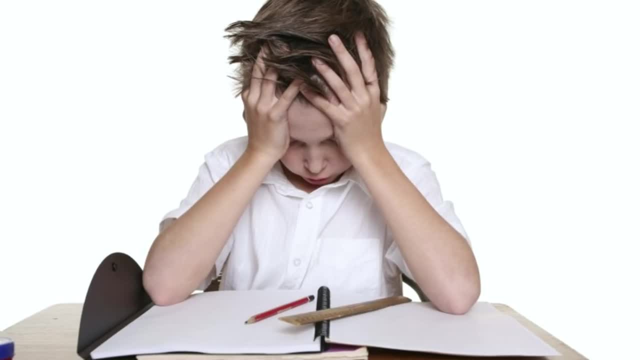 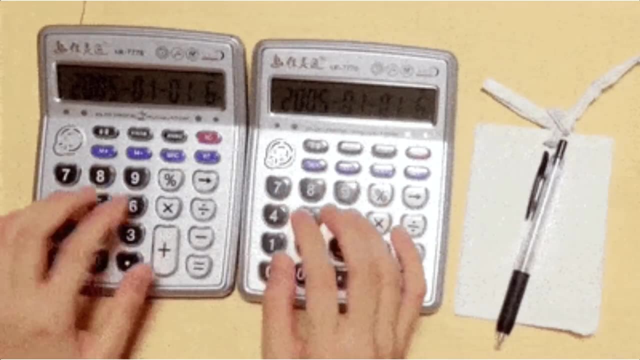 That I don't even know in the first place. So what work am I gonna show? and even if I did know the answer, Why do I have to show work? if it's a problem I could just type in a calculator, then ain't no reason for me to show work. the calculator is my work.